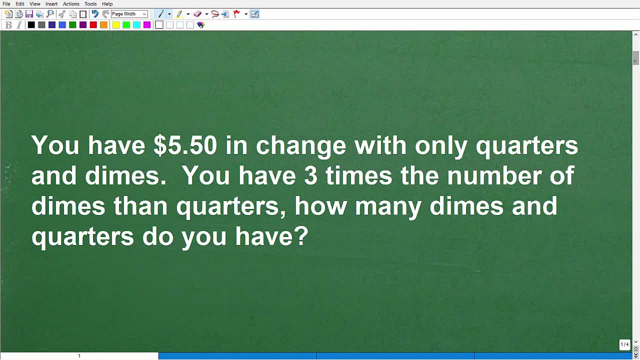 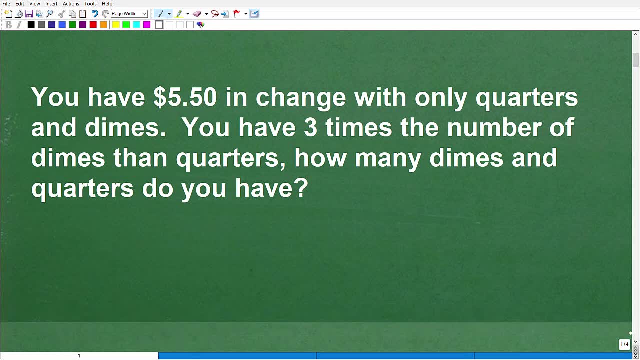 Okay. so first thing about solving word problems like this is what we need to do is to identify a variable. Okay, of course, I already have this work written out, So we're going to you know, see the solution. But what you want to do is say, okay, in algebra we use variables like x and y, etc. So you're going to have to use the information that you have, right. So let's just take a look at some some some things that we know. All right, so we have this value: $5.50.. Then we have this piece of information: three times the number of dimes and quarters, And then, obviously, 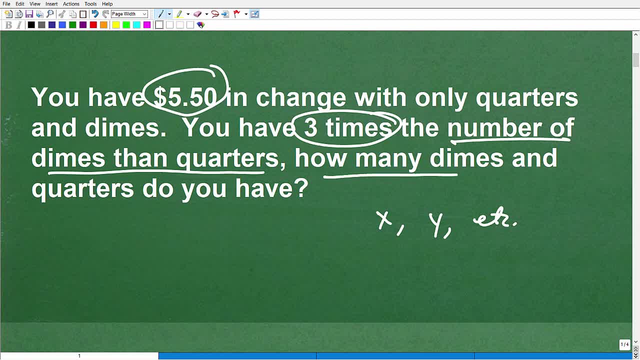 we're looking for two pieces of information: How many dimes and quarters do we have? So what we're trying to identify is how many, okay, dimes and quarters, right, That's. that's the key question. So you have to look at the information you're given and then think about some sort of variable. Okay, we're going to use the variable x. Okay, and what could x stand for? Right, Let's just think about that. What could x stand for? What could it represent? 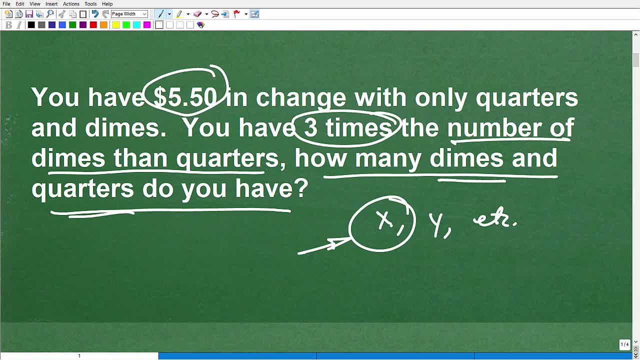 As a starting point in this problem, Okay. Now, once you've kind of determined that, okay, what the whole idea of algebra and a problem like this is, to use all the information you have to build an equation. So first of all, we're going to have to identify a variable, Okay, And then we're going to have to construct an equation, All right. So you know, we're going to have to put some algebra stuff here, some variables, and then it's going to equal to something else. Okay, we have to get to that point. 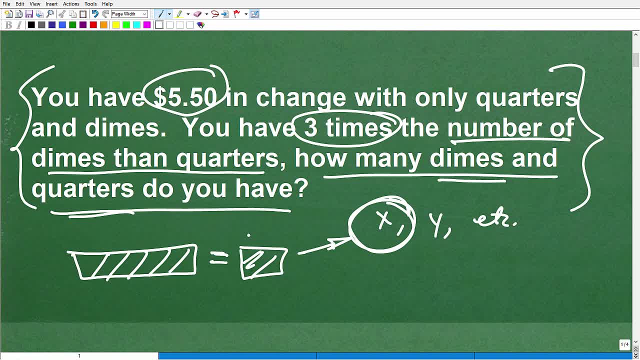 If we can't get to an equation from this information, then we're not going to be able to solve the problem. So once we do have an equation, we can solve for x, for example, and then solve, then solve the problem. Okay, so you can kind of think here like if you solve for x, if you had an equation that was made up of x, what could x represent? Okay, so such that you solved it. you know it could represent something. So maybe you know we're looking for how many dimes and quarters. 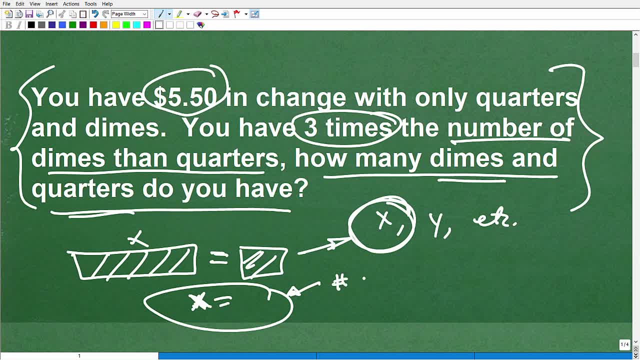 Maybe x would represent the number of quarters you have, or maybe the number of dimes you have, Right, So that would be useful, And in fact that's how we're going to construct the solution to this problem. Okay, so here we go. 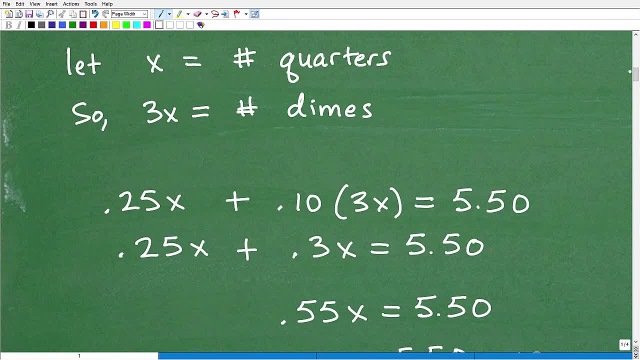 So, without further ado, what we're going to do is let x equal the number of quarters. All right, So x is going to equal the number of quarters. Okay, we're going to only use one variable: the number of dimes than quarters. So if we have X quarters, then we have 3X dimes. Okay, So you. 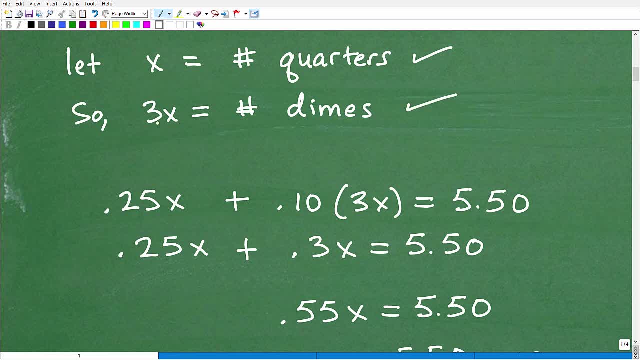 understand that. So if I have whatever amount- because I have three times the number of dimes and quarters, So whatever amount of quarters I have, I'm going to have to have 3X amount of dimes. Okay, So this is the number of quarters and dimes that we have based upon the given. 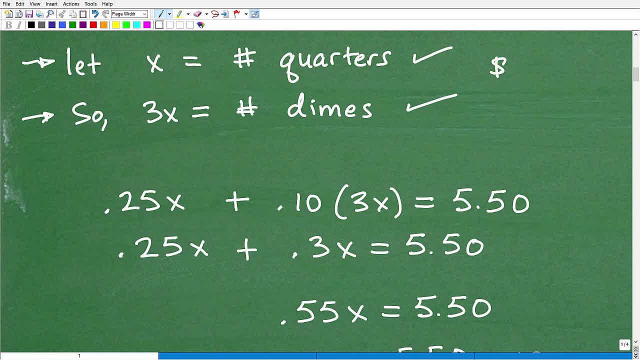 information, Okay, But we have this dollar value, this $5.50.. That has nothing to do with the number. It has to do with the monetary value: how much total money you have. Okay, Not the numbers. We can't construct an equation. Some of you out there might do this mistake. You might. 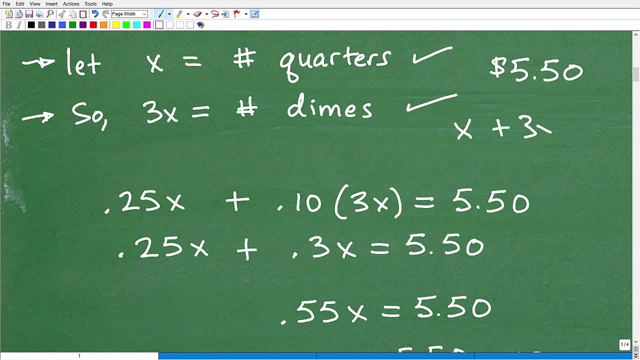 like: oh okay, X quarters plus 3X dimes is going to be equal to 550.. All right, A lot of you would make that mistake, I'm sure, because that's another Quote unquote, classic mistake with these type of problems. But in fact this is not the case. 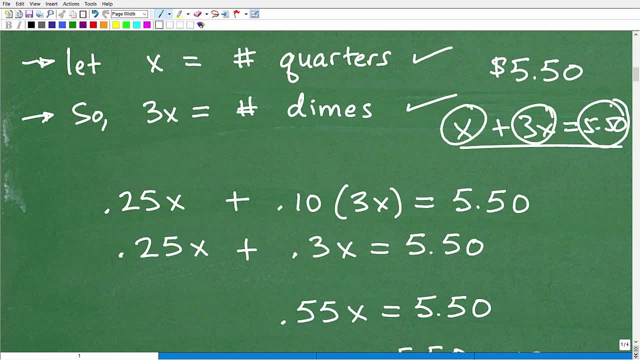 This is how many quarters and dimes you have. That's not going to be. you know, you can't write it like this. from a monetary standpoint, We have to give the values, because this is dollars, right, This is $5.50.. So quarters and dimes have different values, So we have to account for that. 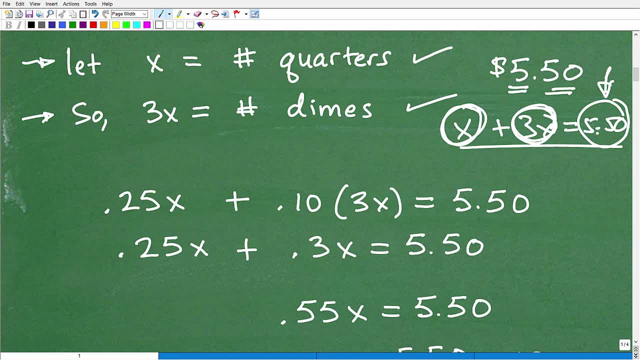 in this equation. So a quarter is going to be 0.25.. X. okay, of how many the number of quarters you have. Okay, So if I have one quarter I would have 0.25 times one, or just 25 cents, Okay. So again these problems, once you figure out how to do one. 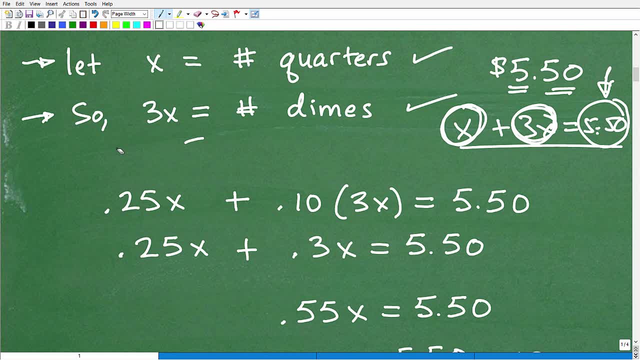 and you come across a money problem like this again, something that deals with money and quarters and dimes, you know again, very classic, In other words, these type of problems show up frequently. So once you figure out how to do one, then you can get that main idea. You can do others as well. 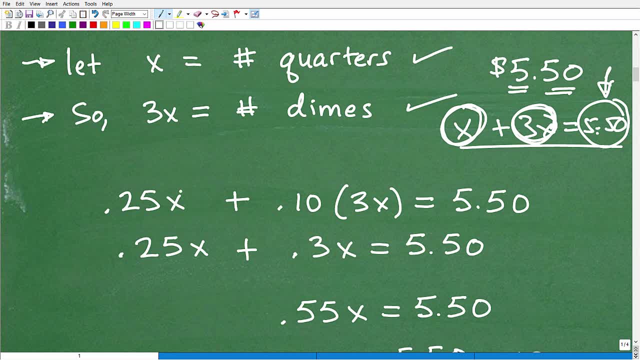 All right, So here we go. So 0.25 X, this is our quarter value plus the value for a dime is 10 cents, right? So that's going to be 0.10 of a dollar, because we have $5.50.. Now X is the number. 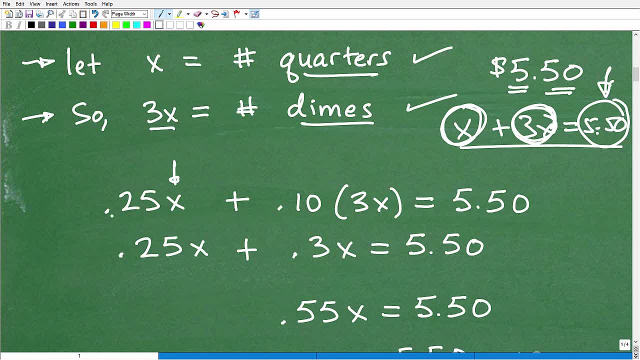 of quarters we have, and three X is the number of dimes. So it's going to be 0.25 X plus 0.10 zero. Okay, This is the value of the dime times the number of dimes we have, which is three X. 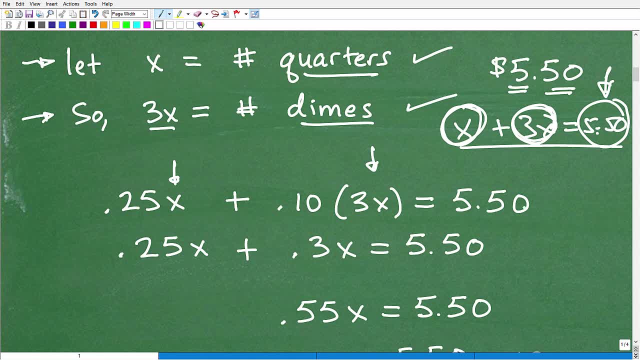 And that is going to be equal to $5.50.. Okay, We don't have to write the dollar sign, dollar value in here, because you know we're not, we're, we're setting up an equation, Okay, But you know. 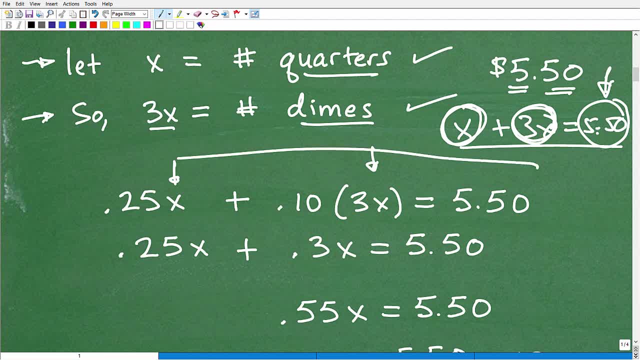 what it represents. All right, So at this point, the most important part of this problem, up to this stage of it, is to get the equation right. Okay, So the first thing is pick a variable, let's say X, And if you're confused about what that variable should be, 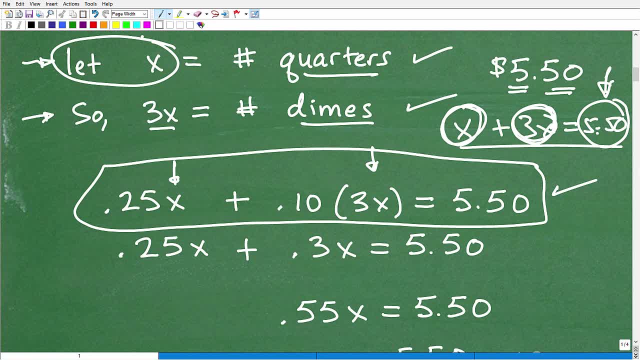 think about what the question is asking. Okay, So we want to know the number of quarters and dimes, right? So let's let X equal, for example, in this case the number of quarters, and then we can kind of build another expression: number of dimes. Now we have to put all the given. 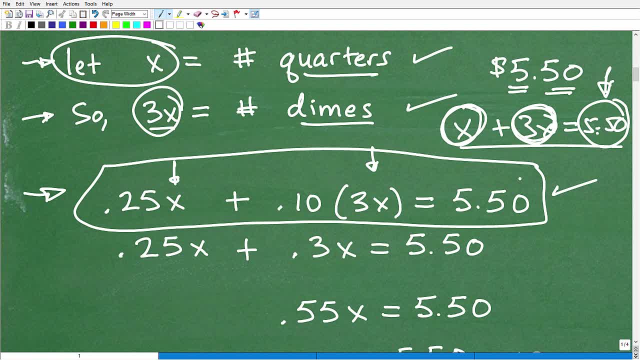 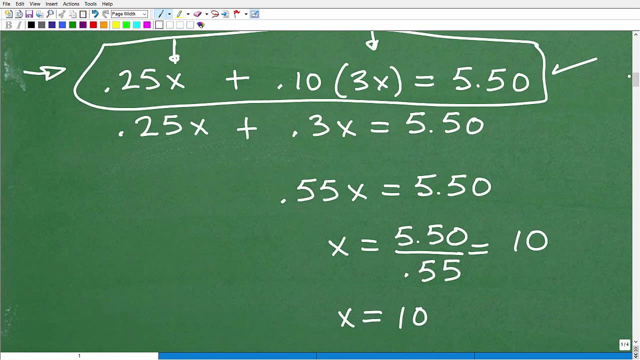 information into. we have to put it together in form, in a, in terms of a, an equation. Okay, So double check. Hey, this makes sense. This makes sense. Now, at this point, you can go ahead and apply your outstanding algebra solving skills. All right To solve for X. So we got 0.25X plus. 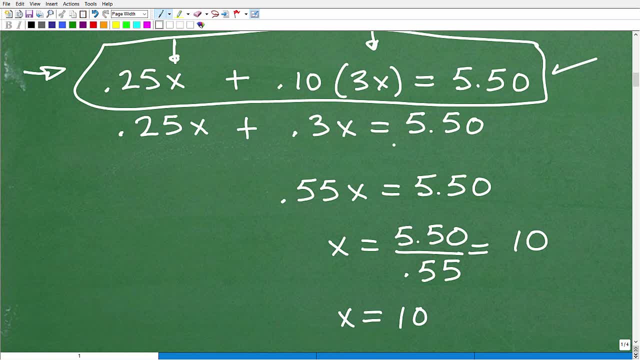 0.10 times 3X is going to be 0.3X- And you can use a calculator to help you out here- And that's equal to $5.50.. And then, when we add these two terms up, 0.25X plus 0.3X is going to. 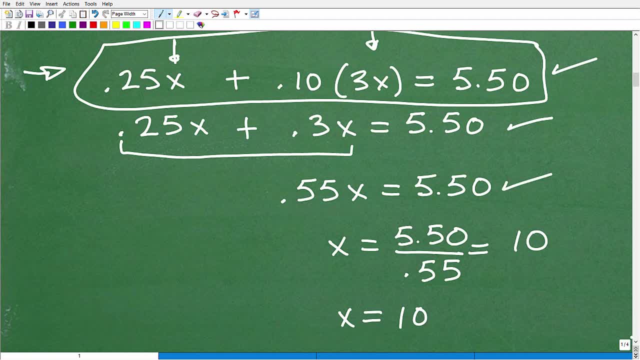 be 0.55X is equal to $5.50.. And then, when we add these two terms up, 0.25X plus 0.3X is going to be 0.5X, And then we're going to divide both sides of the equation by 0.55.. Okay, So this is we're. 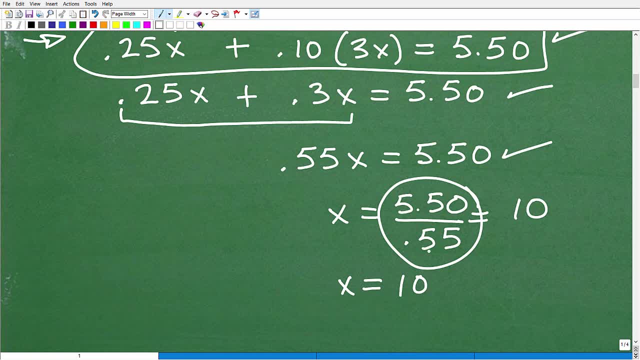 going to end up having, and so we got 0.5X divided by 0.55.. You get X is equal to 10.. So there you go, You got a nice solution. You have X is equal to 10, but what does that mean? Okay, Well, what? 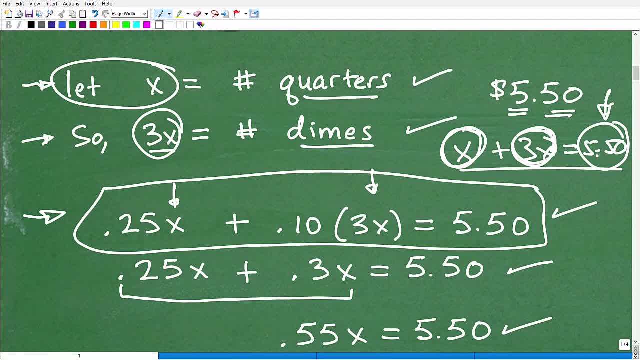 was X again. You have to go back up here. Remember we were saying that we're going to X, equal the number of quarters. So X is equal to 10.. So we have 10 quarters. Okay, So if we have 10 quarters and we have three times the number of dimes and quarters, then we have 30. 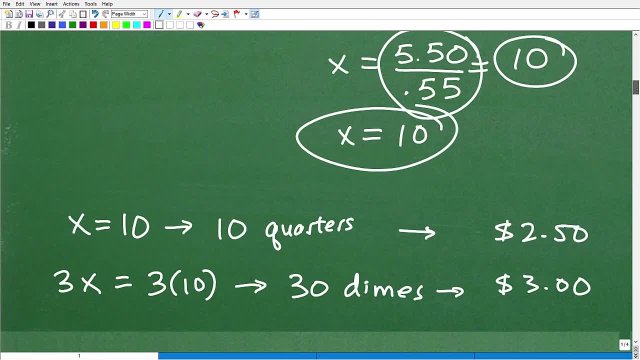 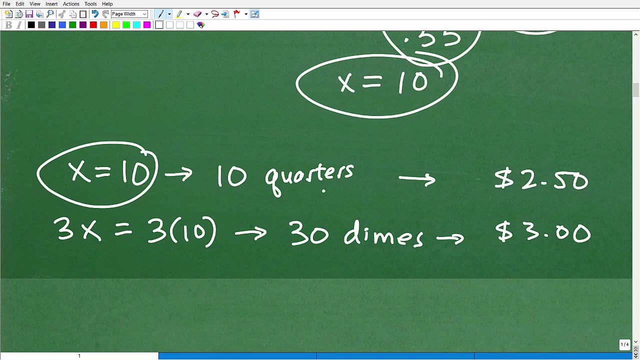 dimes, right? So let's go down here. So X was the number of quarters, So we have 10 quarters. So 10 quarters, right, is how much? in monetary value, That would be 10 times 0.25, or you would. 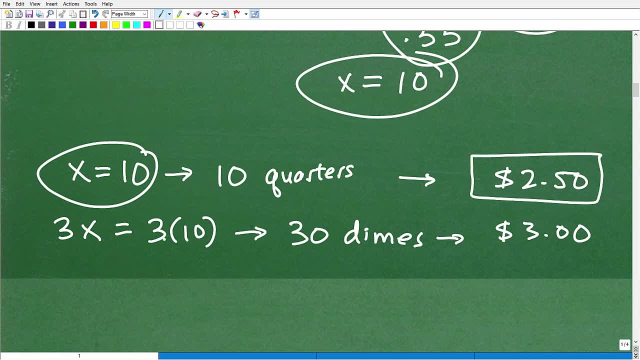 have $2.50 worth of quarters, but you have three times the number of quarters. You have three times the dimes. You have three times the number of dimes, Then quarters. Hopefully I'm saying that right, I'm not confusing myself. But what we're saying 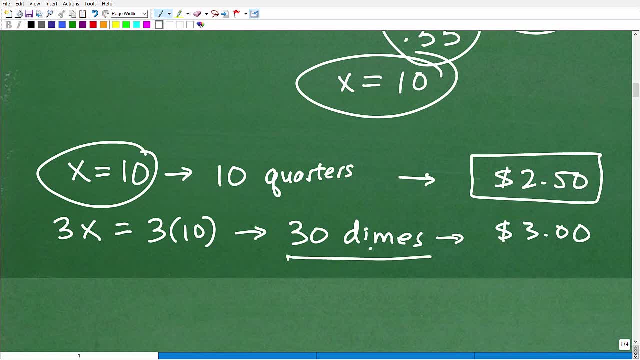 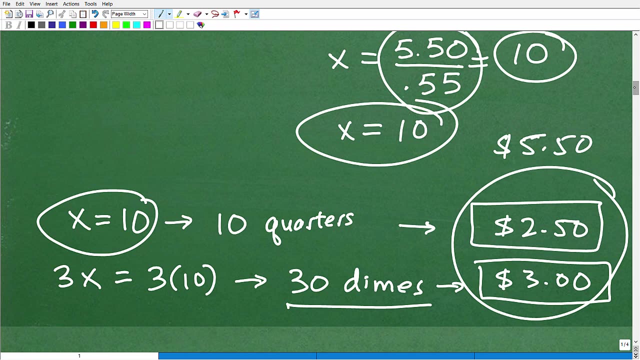 here is: we have 30 dimes, right. Three times the number of dimes and quarters, right, We have 30 dimes and a monetary value of 30 times is equal to three bucks, And if you add this together we get back to our $5.50, right? And that's what we have in total. Okay, So classic algebra word. 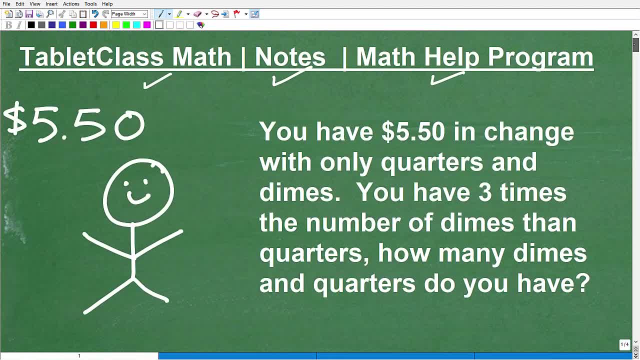 problem Just as fun as anything. You may attempt the rest of your day here. I mean, this is good stuff, You know. you get asked you know, when am I going to use algebra? I'm never going to use algebra, now You know. 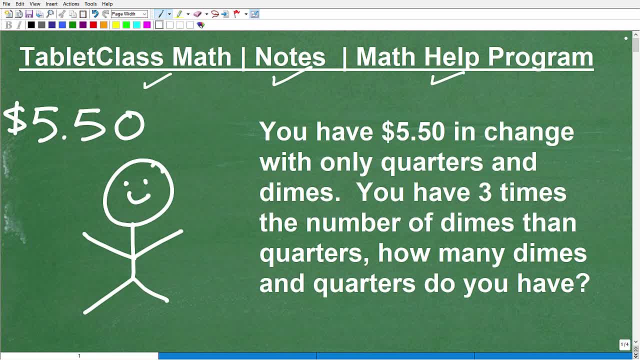 is this a practical problem? No, but it's a fun problem And it's an illustration of how we do solve word problems using algebra. Okay, But believe me when I tell you you know algebra is used in real life. Okay, Outside the classroom it's absolutely used to solve problems.